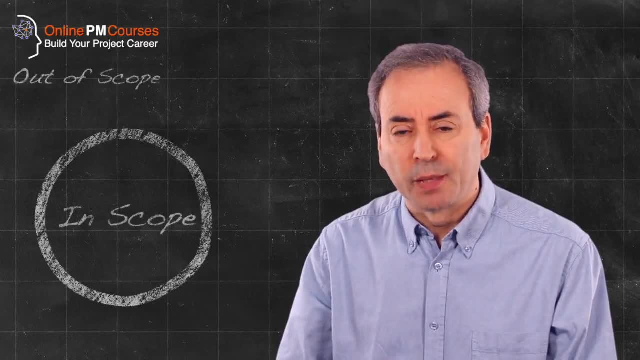 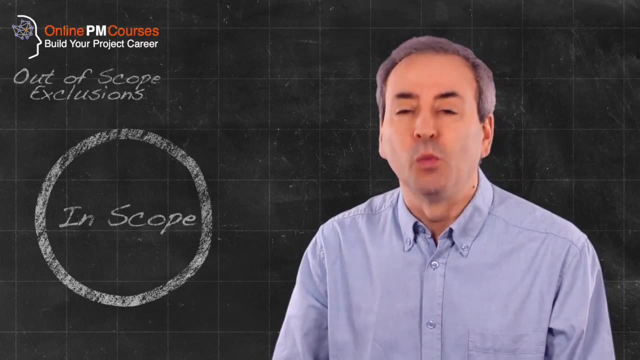 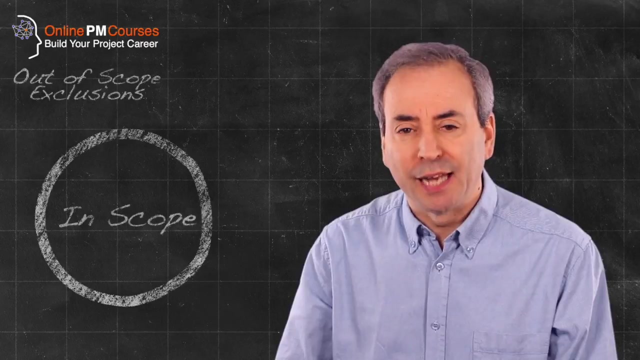 So if everything inside the circle is in scope and everything outside the circle is out of scope, sometimes called project exclusions or exclusions from scope- what's the issue? The issue, of course, is stakeholders, try to feed additional functionality into your scope. 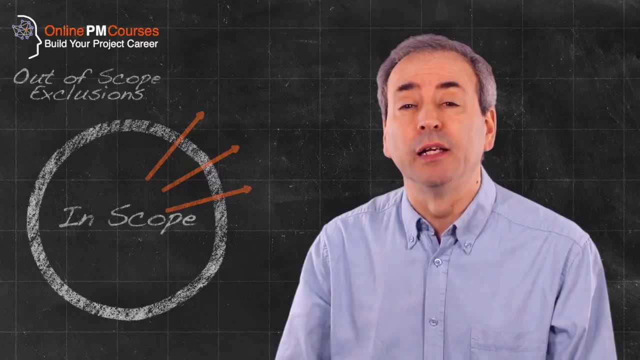 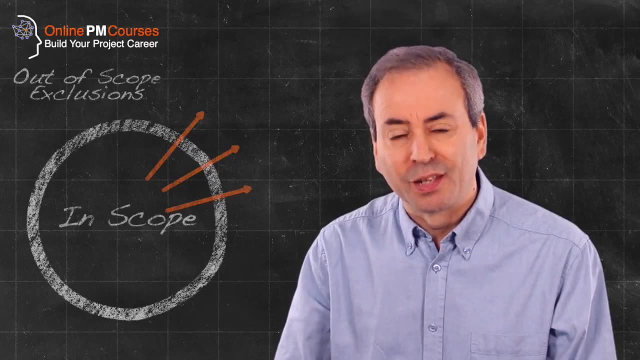 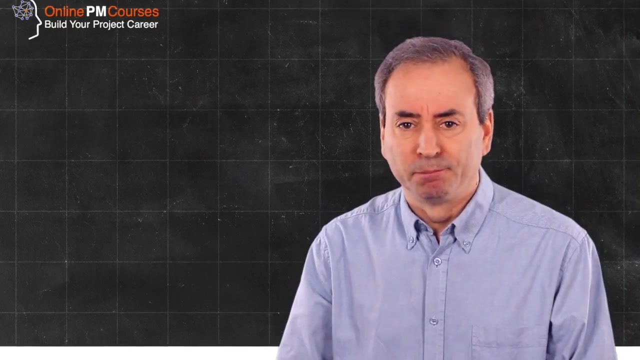 therefore extending the scope boundaries without necessarily increasing your resources or your budget or your schedule to allow for you to deliver them. This is known as scope creep. So why is negotiating scope so difficult? Well, the answer is simple: because you've got many. 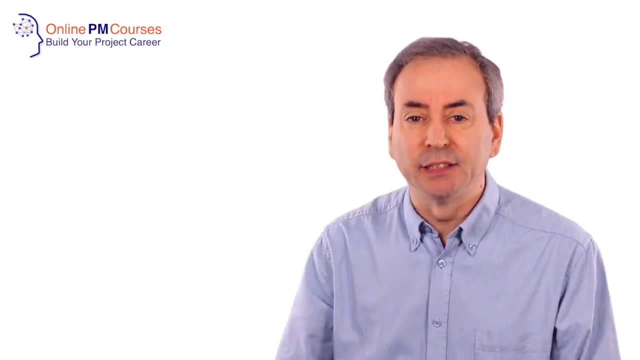 stakeholders. You've got a lot of stakeholders. You've got a lot of stakeholders. You've got a, And each of them has different preferences, different needs, different wants, different desires. They have different agendas and different interests And the process of negotiating scope. 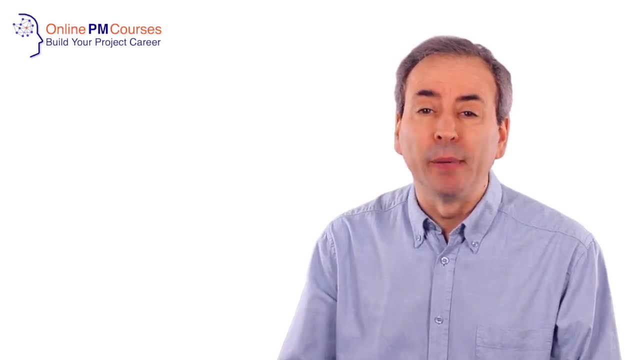 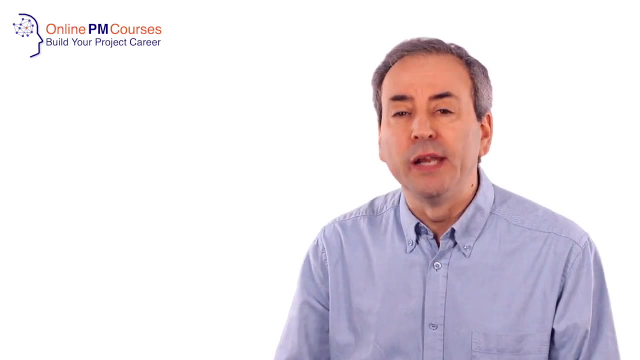 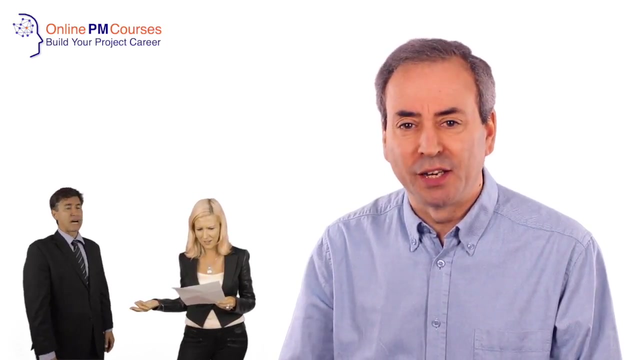 is negotiating against all of those competing pressures, trying to satisfy this person and that person at the same time, and all of this with a limitation on the resources you have available. So it's a multi-way negotiation, with different stakeholders trying to negotiate and balance among their different needs and desires. 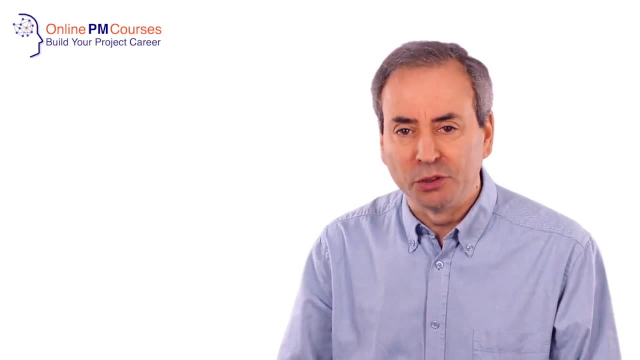 And, of course, with other stakeholders negotiating for additional resources or additional time in order to deliver the greater amount of scope. Consequently, you won't please everybody. Your job as a project manager is to find the best balance that you can to satisfy and smooth over the concerns of as many stakeholders as you can. 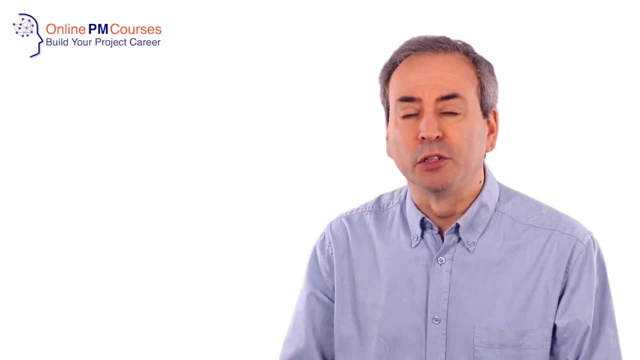 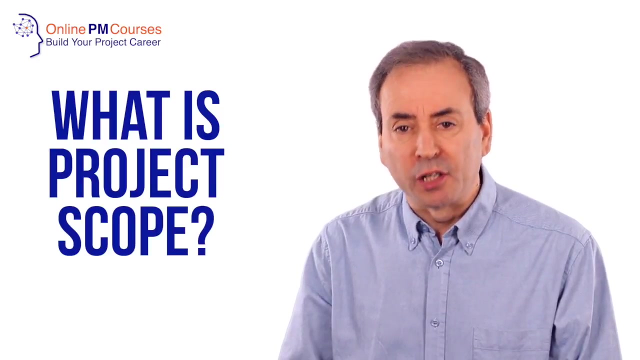 and to get it signed off, And you can do that by those stakeholders who have the ultimate authority to decide what the final scope will be, what the final budget will be and how long you have to deliver it. So scope is an easy concept, but negotiating it and documenting it and making it stick. 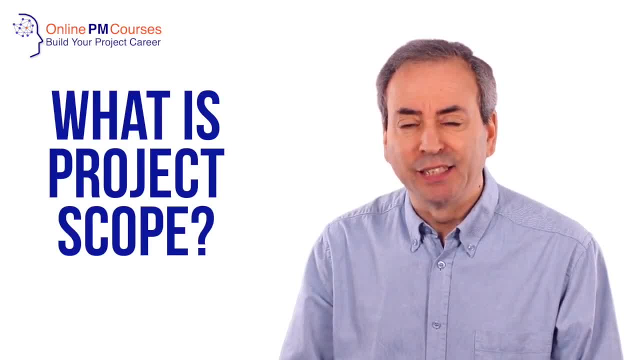 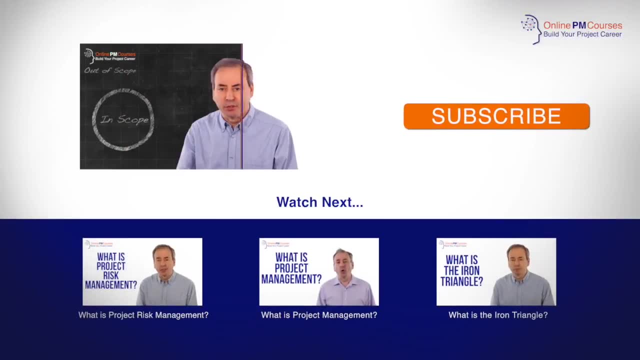 and winning over your stakeholders at the same time is a tremendously difficult challenge For me, the very hardest we face as project managers. Subtitles by the Amaraorg community.